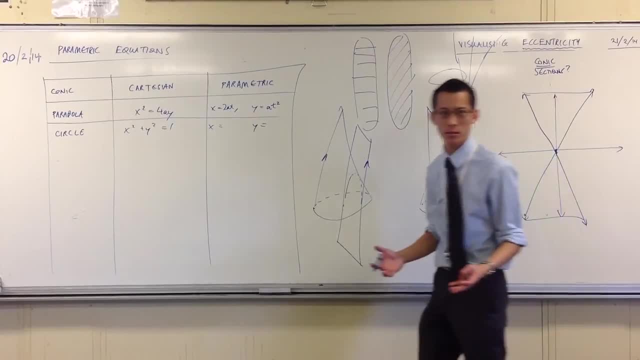 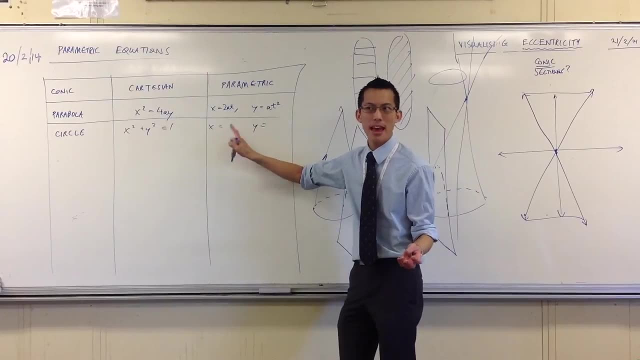 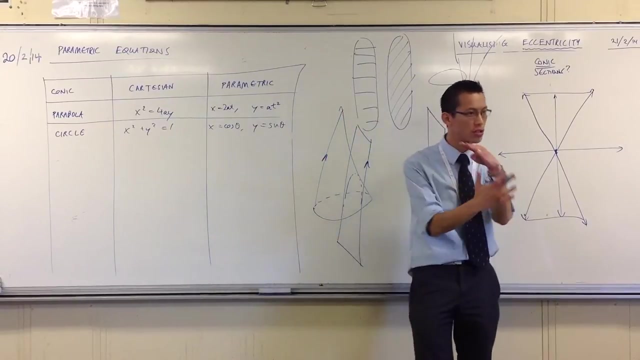 What were the coordinates? It was a trig thing, wasn't it? It's sine and cos, but which one's which x is cos? and the way I remember it is, it's alphabetical, And that makes y sine. And of course you can draw the unit circle for yourself. 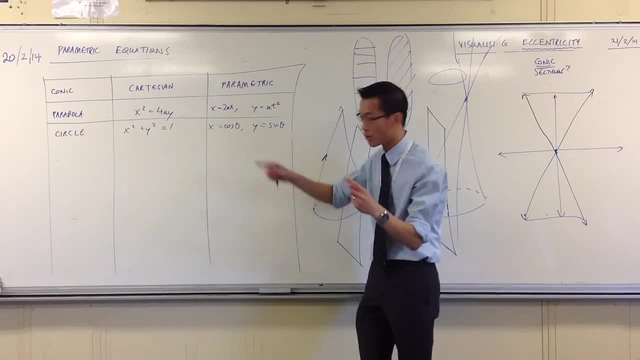 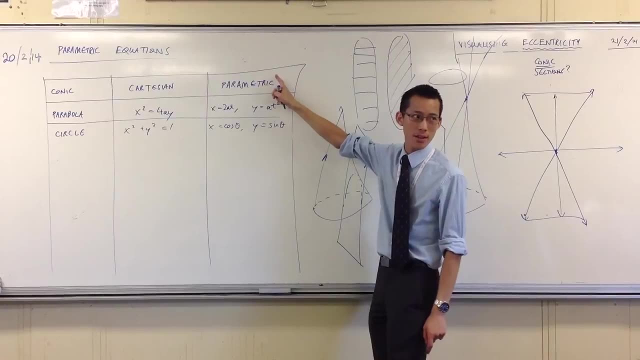 And you'll see, college refers to that horizontal distance, Hence x, And sine refers to the vertical distance, It's y. Now we actually gave it a different name. Do you remember what we called it? We didn't call it a parametric equation. 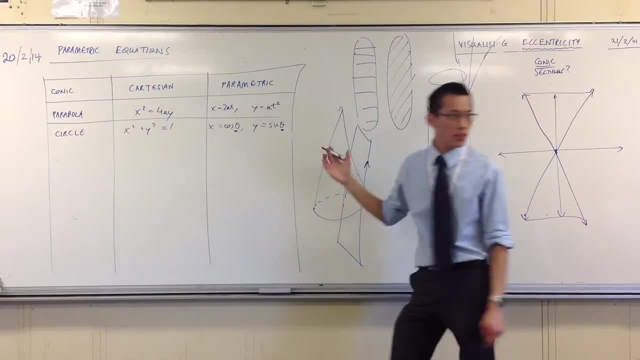 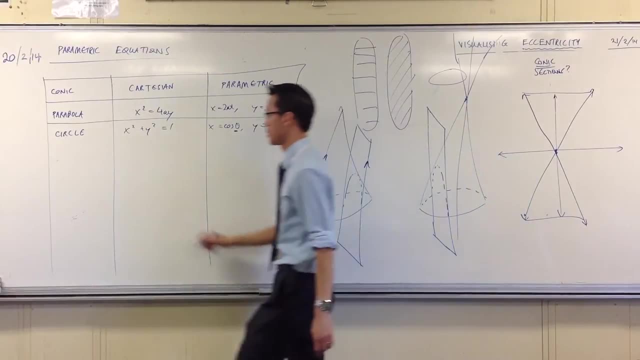 Because it has to do with this angle. we often called them polar coordinates, Because that defines things in terms of angle and radius, So we'll revisit that word in a second. Now, if that's what a circle is, we know an ellipse is. 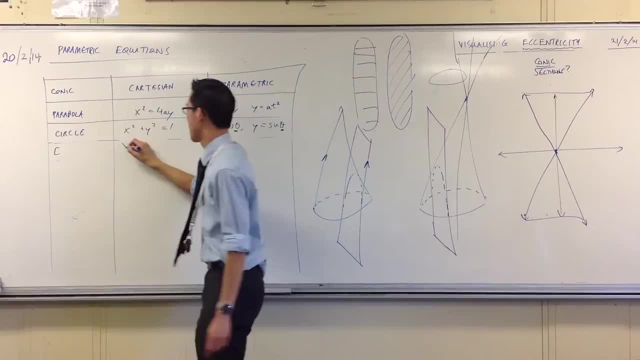 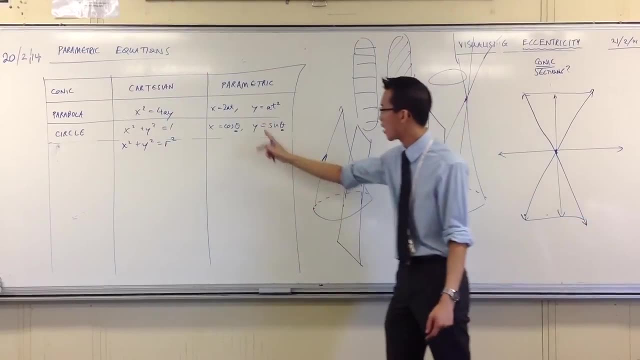 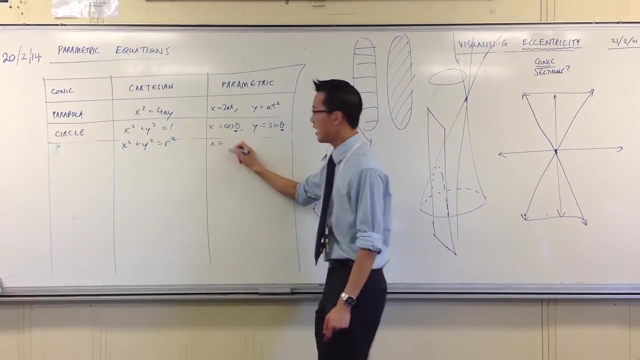 Oh, sorry, I skipped something. Let me generalize That was the unit circle. Let's do a general circle. If all I change is I make the circle bigger, how are the polar coordinates, the parametric equations, how are they going to change? 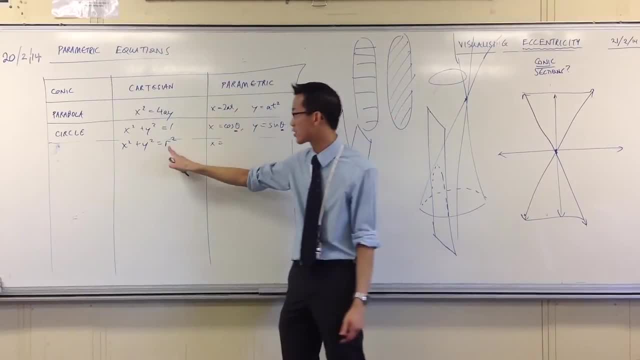 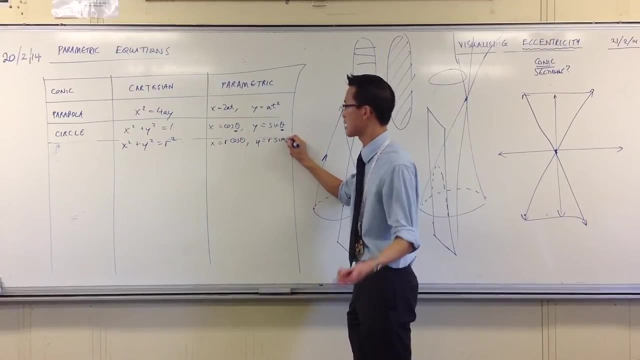 Well, they're going to get further out, further away from the origin, by a factor of the radius. So that's going to be r cos theta and this will be r sine theta, And that's the only difference. Now I can move on to the ellipse. 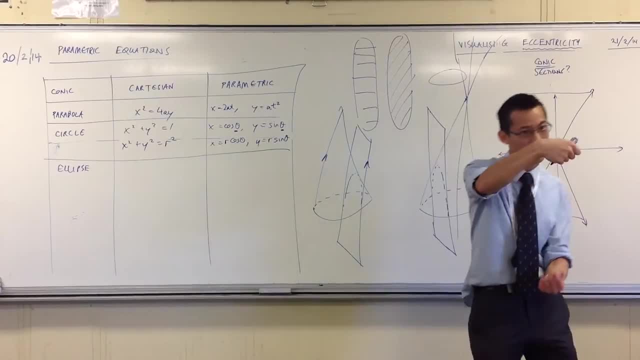 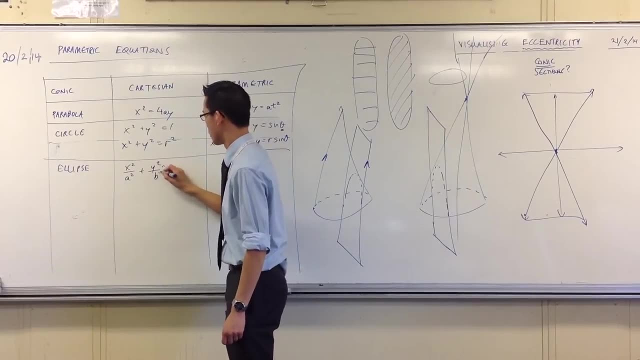 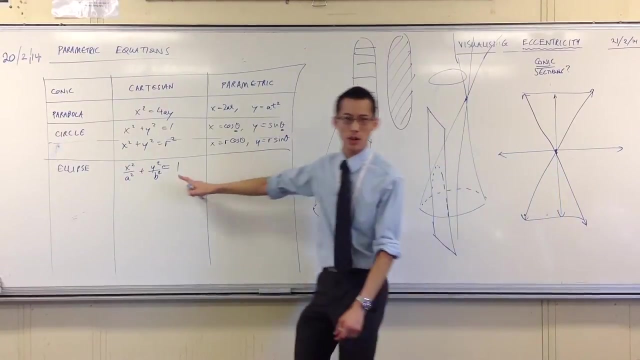 Now being that an ellipse is just a circle that's been stretched out in different ways. If we consider the basic one, which has its center at the origin, The nice thing about this equation is it's already got its proportions built into it, based on a and b. 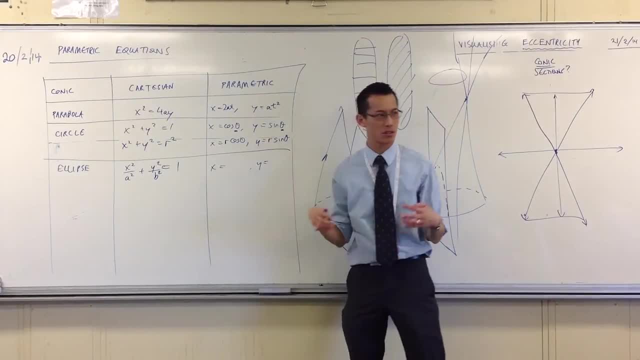 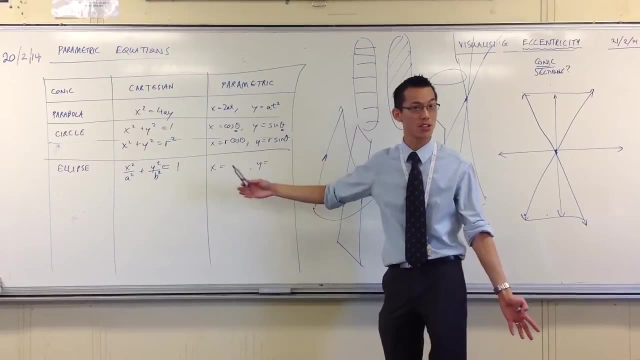 Intuition kind of tells you: well, the cos and sine things should still sort of be happening, Right, Because it's still going around and around in the same way. And these are the. They're also called circular functions, if you remember that. 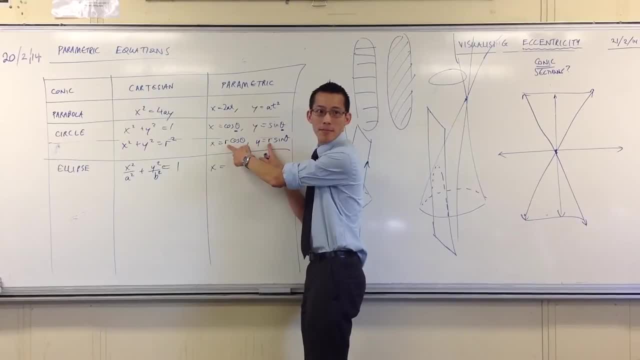 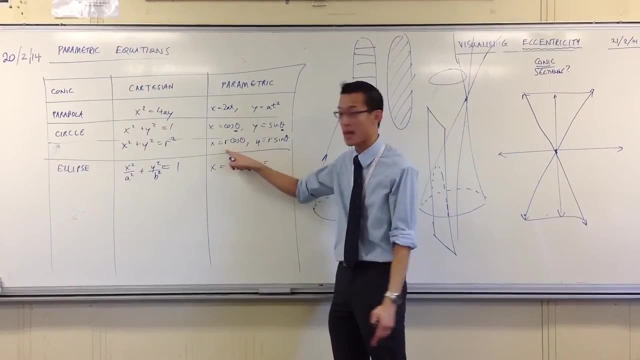 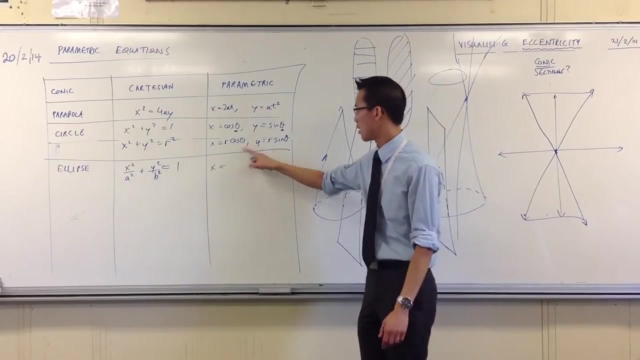 But they're not going to go around and around in this neat way, This equal way Right- Sometimes you'll be further across than you are high- rather than exactly the same amount. So how do we account for that? Well, how do we get r cos, theta and r sine? 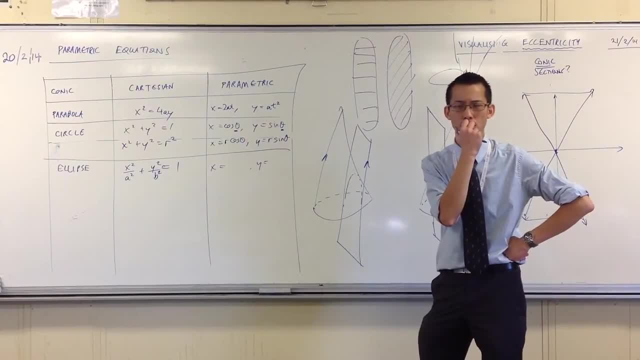 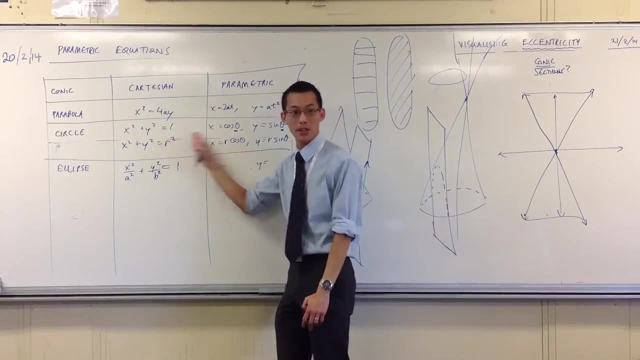 Why do we multiply by r? Why do we do that? Change the radius, Change the radius Right. We know that, for instance, if r was 5,, 25, we're just going to be the same things but further away. 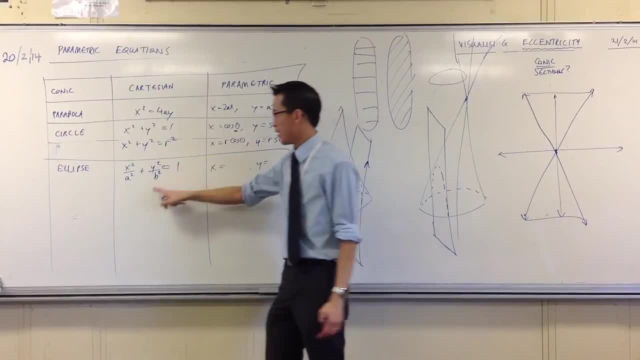 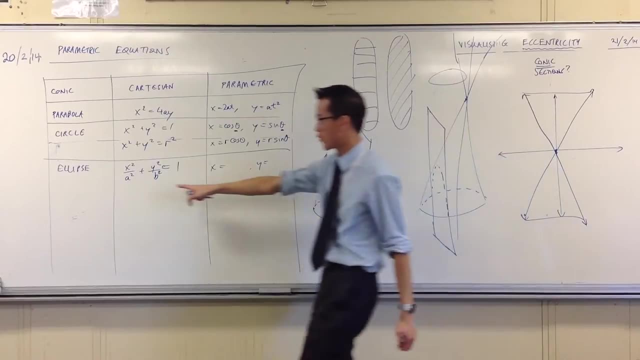 And how much further away was the radius. Now, a squared and b squared are how much further away you are horizontally or vertically, Because if I make this a really big number and this a small number, that makes you really fat, or vice versa. 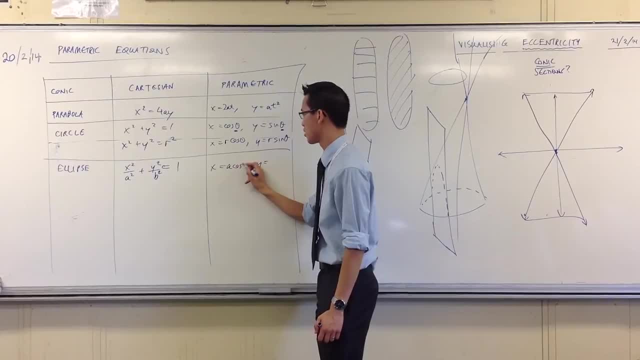 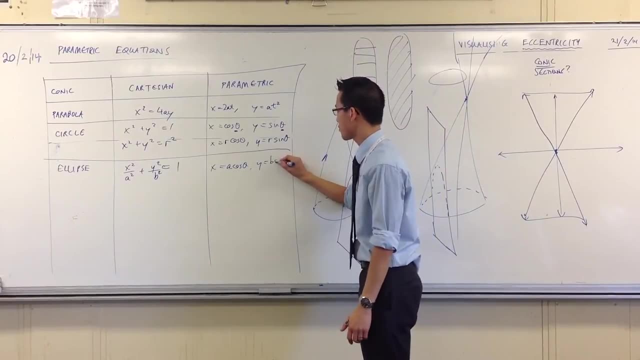 So therefore, instead of r cos theta, you're just going to have a cos theta. That's how far across you can go. Right, a is what defines how wide your ellipse will be And, in the same way, because y is operating on a completely different system, based on how tall or squat you're making it. 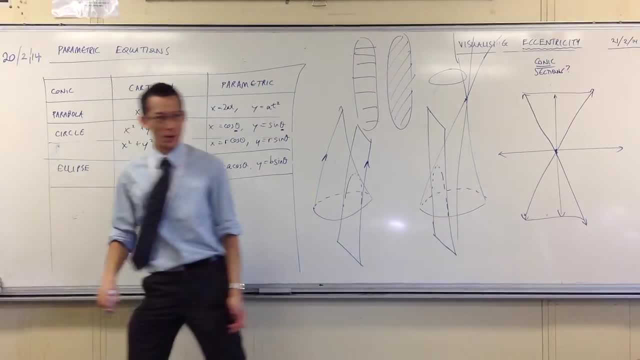 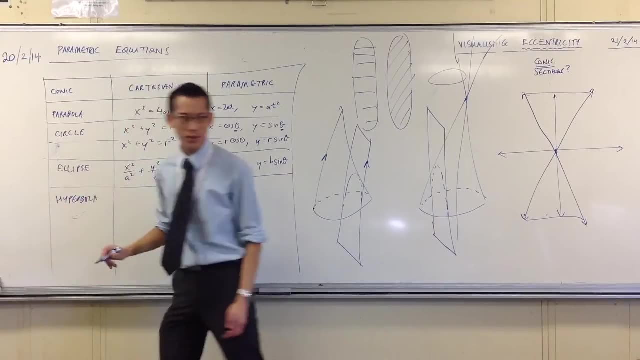 it'll be b sine theta. Right now we have one last conic section. what we've done today? Now we sort of did some logic and the proofs, geometrically, are very, very simple. for all of these, The hyperbola is not so neat. 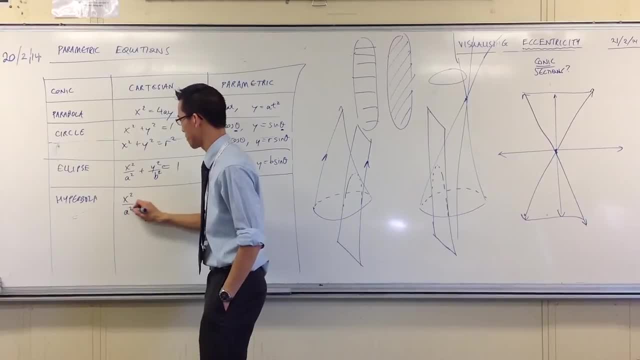 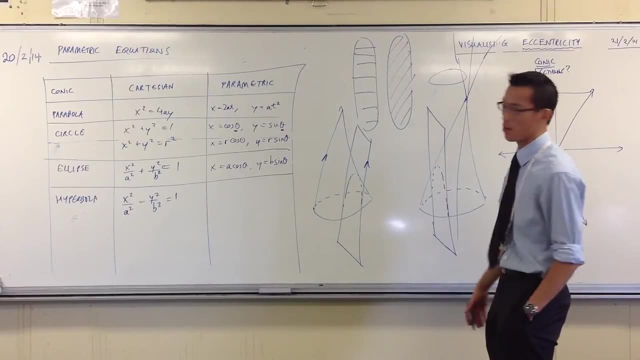 Okay. So what I'm going to do is I will give you the parametric equations, Okay, And we're just going to show that they work, But I'm not going to derive the actual results for you, because they will take you forever. 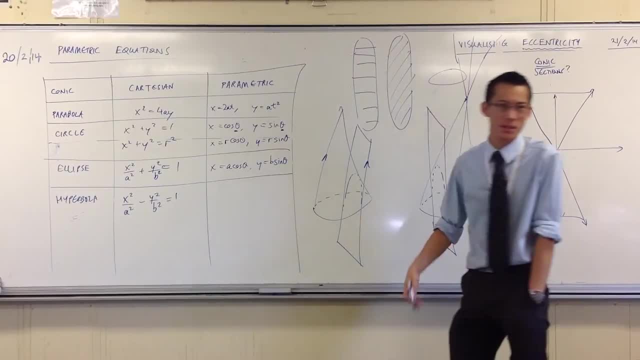 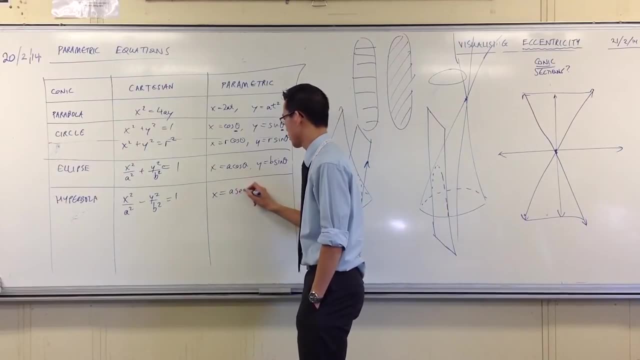 And you won't gain that much out of it really. It's just your head sort of spins with intrigue and it's confusing. Okay, So we're going to go like so And I think from memory this should be: sec theta. ny equals tan theta. 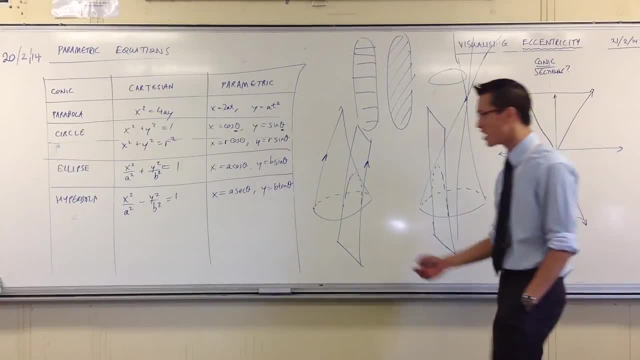 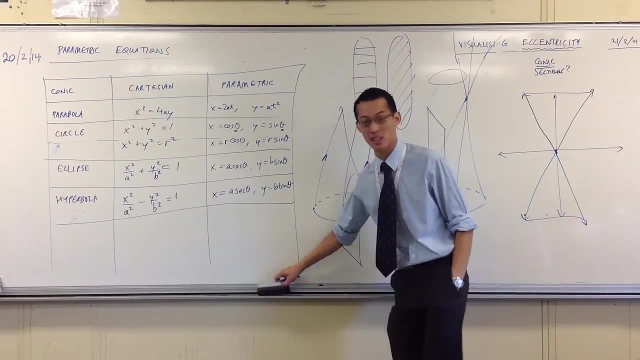 Is that about right? Good, okay. And you're like: hmm, where does that come from? And the answer is: some wacko geometry. But let's just quickly make ourselves content that this works And it's a very, very simple trig identity that will let us do it. 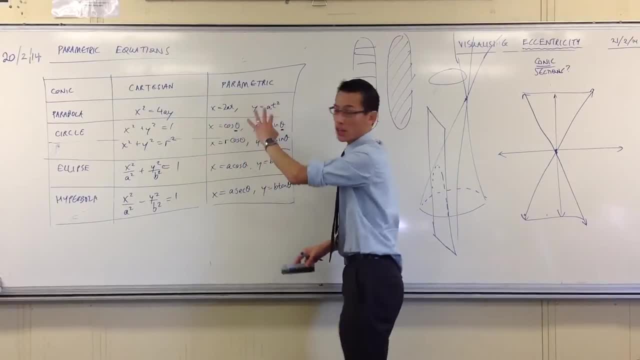 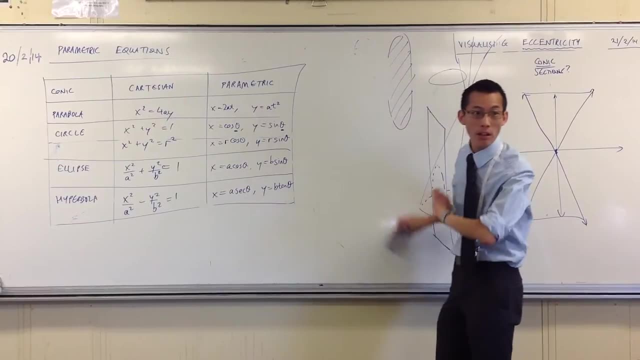 Okay, What were we saying at the beginning? The parametric equations. when you stick them together, you should get the Cartesian equation Right. So, because I've got expressions for x and y, all I have to do is sub them in and let's see what happens. 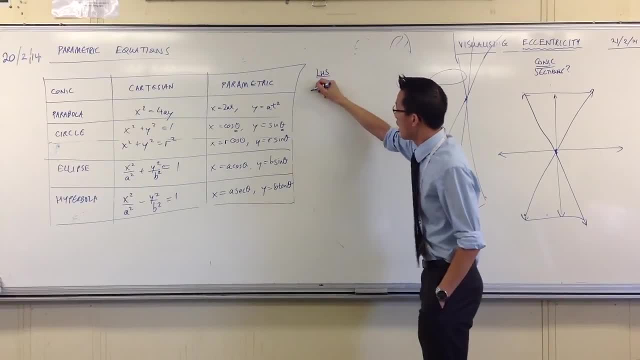 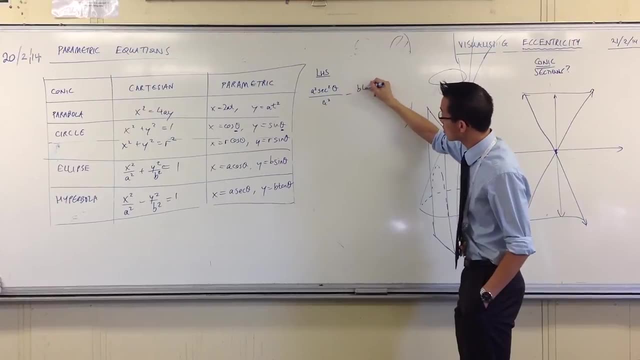 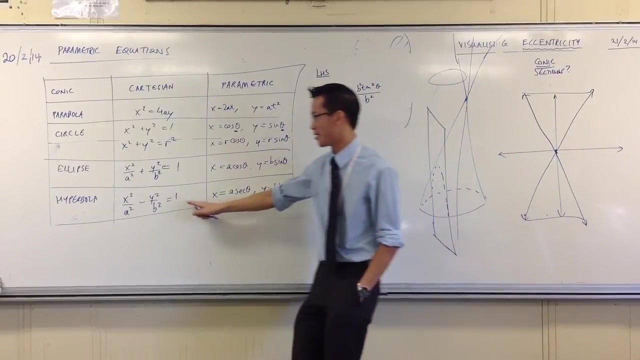 So I'll take the left-hand side. I'm going to have, let's see, a squared, sec squared, and b squared, tan squared. That's what I've got. So I know where I want to end, right? So there should be some funky cancelling out here, right? 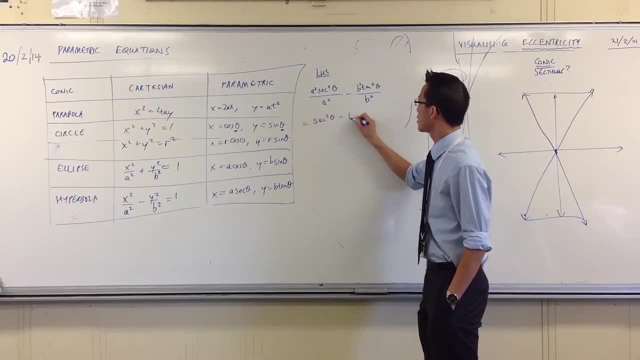 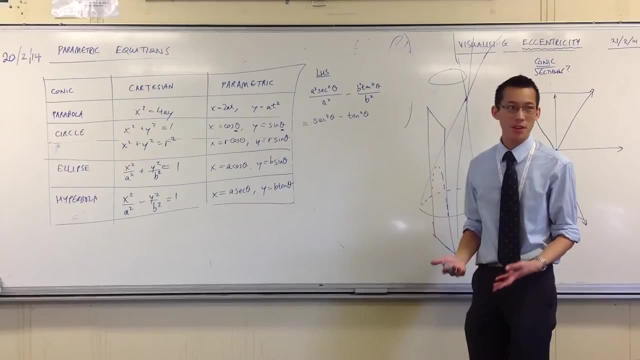 The a squared and the b squared- cancel. That's nice. Now, here you can see sec squared and tan squared. Clearly there's the Pythagorean identity that's going to come into play. Now, I don't know about you, but I always found it a nightmare to try and remember. 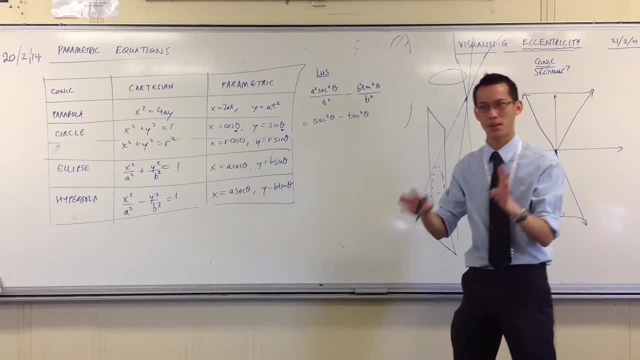 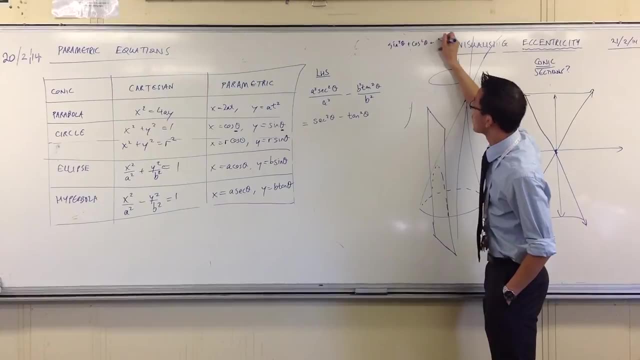 is it 1 minus tan squared, is sec squared or the other way around? I always found that confusing. Okay, So here's the way that I do it. Just go back to the original Sine. squared plus cos squared equals 1.. 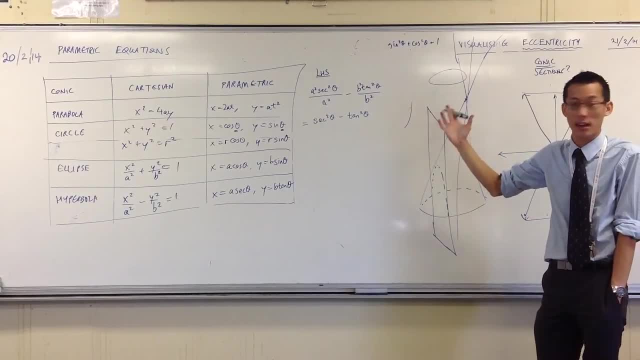 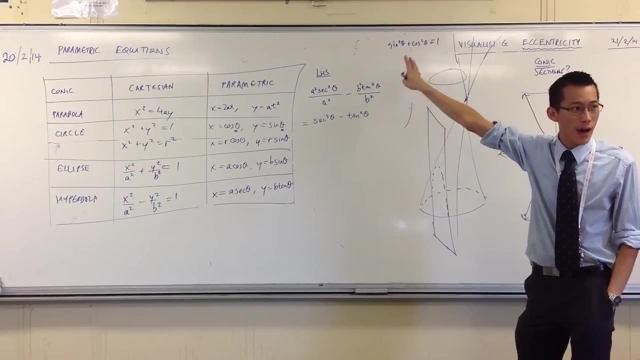 Right, Everyone remembers that People don't seem to have trouble with that, which is great. Okay, How do you go from this one to the one with tans in it? What do we do to everything on that line? You divide by cos squared? 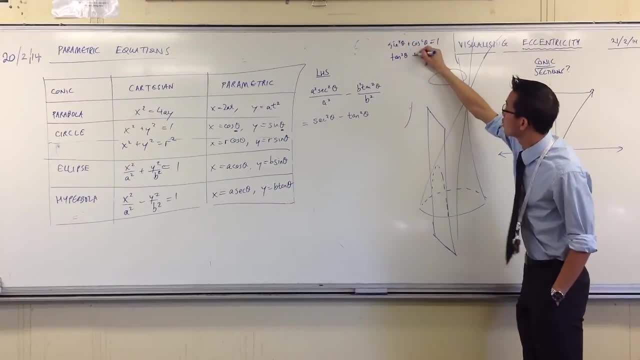 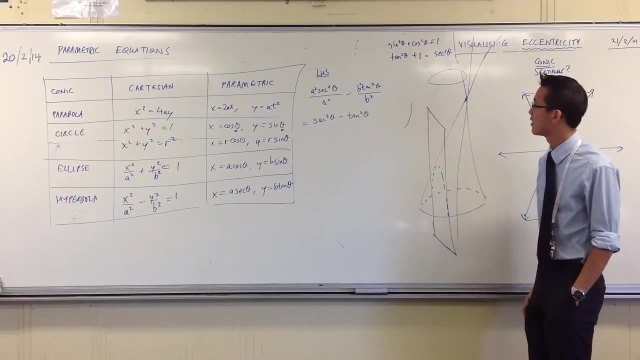 Okay. So divide that one, You get tan squared. Divide this one, You get 1.. And then you have your reciprocal identity along the n. So that's a really nice, foolproof way of never screwing it up. Therefore, I'm going to stick that in there. 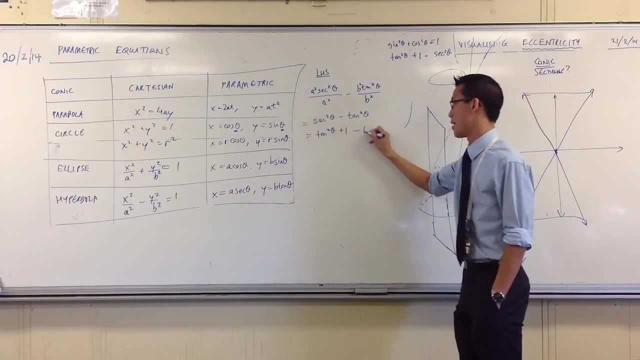 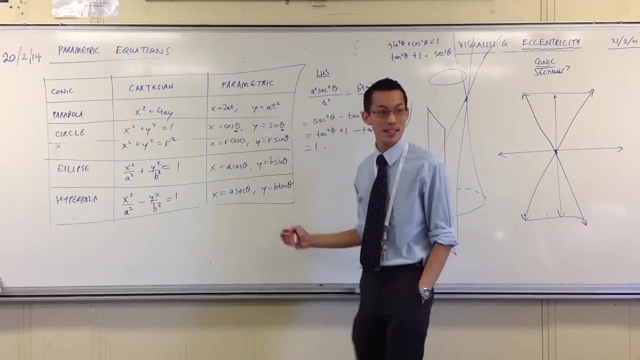 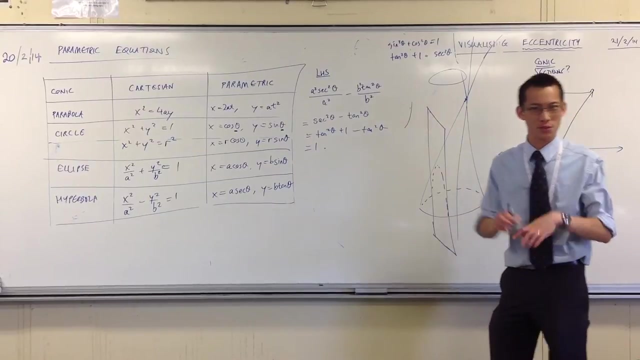 So I get my tan squared plus 1 minus tan squared, which is the one that I was expecting, Thank goodness. Okay, So this works. It does actually satisfy the Cartesian equation. All right, I'm going to look it up, but it's kind of long involved and I don't think it's that beneficial for you guys. 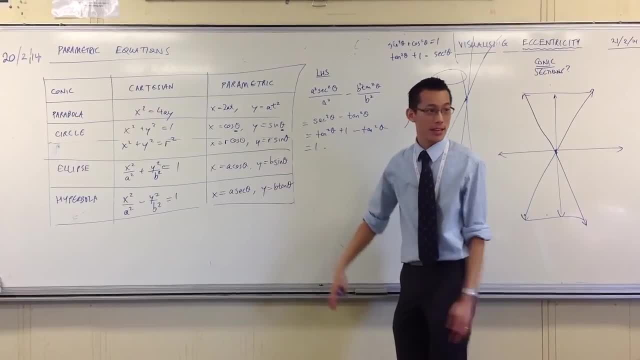 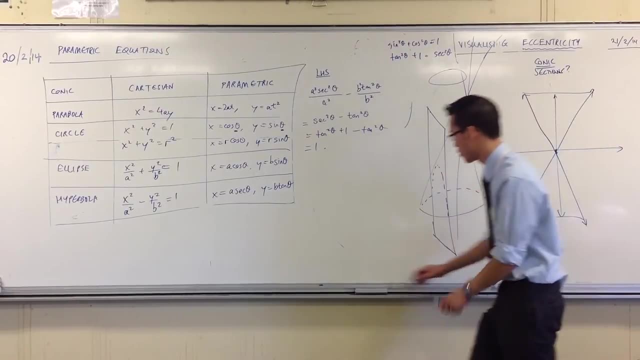 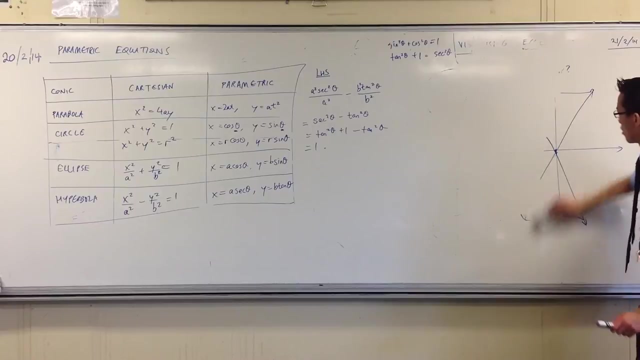 Okay. But here's the point: You can use all of these to solve questions in a way that's a bit easier sometimes and maybe needs less logic, if you like. So let me show you. Go back to one of those questions where you had to prove that the distance from – I'll draw it for you. 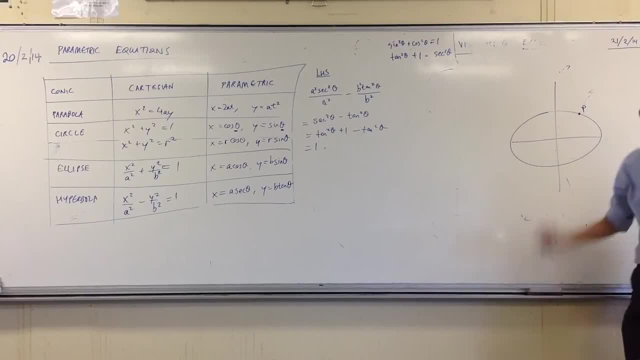 The distance from any point on the ellipse – pick a point, Okay, And draw the distance to the two furcades. Do you remember this? Like here's one focus and there's the other one, So what do we call them? 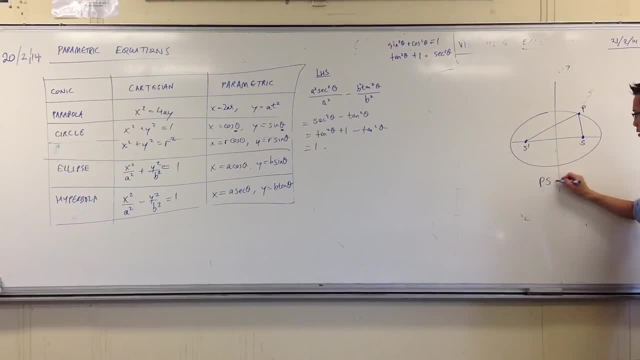 S and S dash. You had to prove this Right. What were they equal to? What was the sum equal to? We wanted to prove that they were equal to the major axis And we did some sort of chopping and changing to do that. 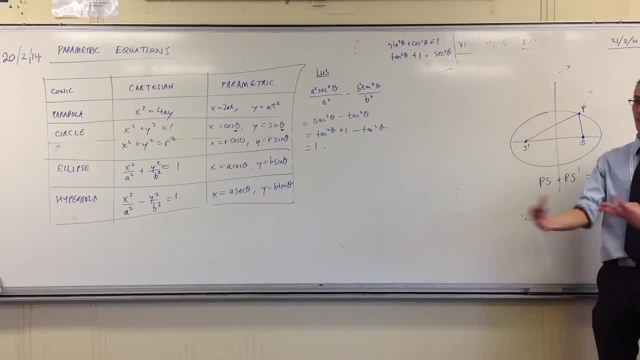 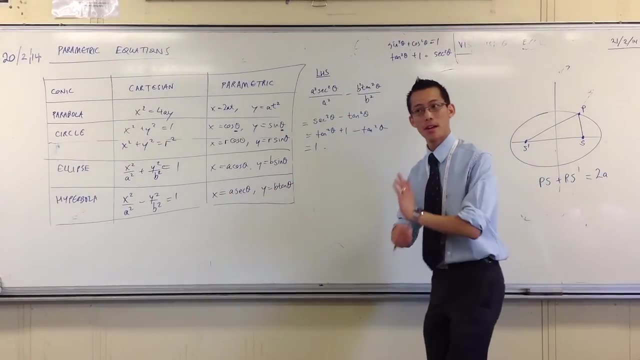 Right, What did we use? We used the Locus definition of the ellipse. blah, blah, blah. Now, if I have exact values for the x's and the y's, it's just algebra Watch, Okay, P S. 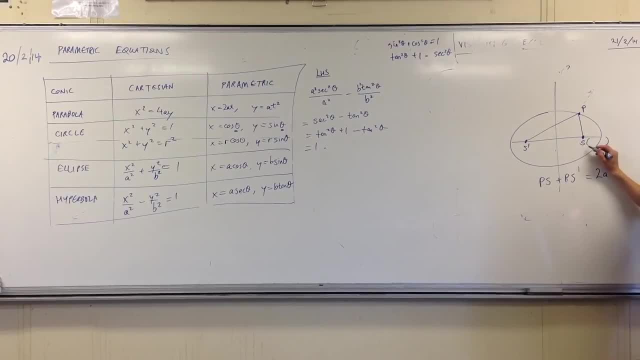 What is S? What are its coordinates, The focus, Where is it? It's A E, isn't it Zero? Okay, And correspondingly, this is minus A E, Zero Okay. So therefore I can just say: well, what is P? S? 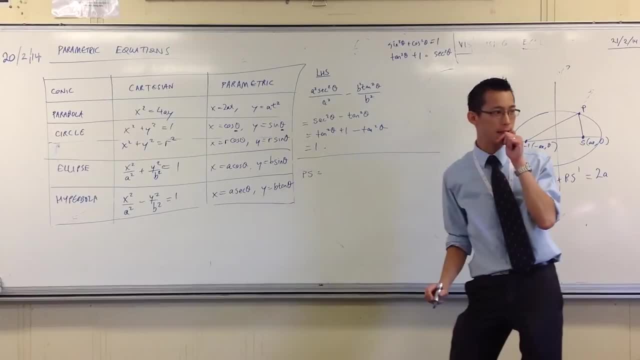 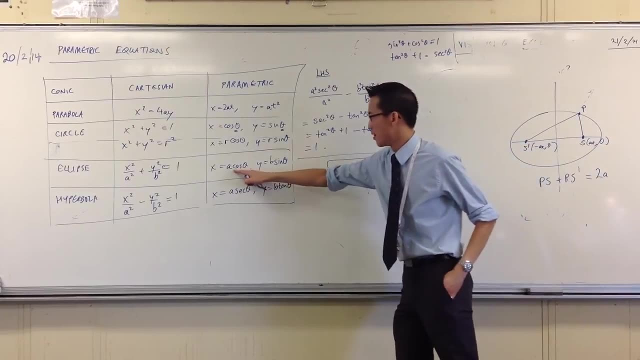 What's it equal to? It's the square root of – well, this is just the distance formula, isn't it? I'm going to go from these coordinates, A, cos, B, sin, and I'm going to go from these coordinates, A, cos, B, sin, and. 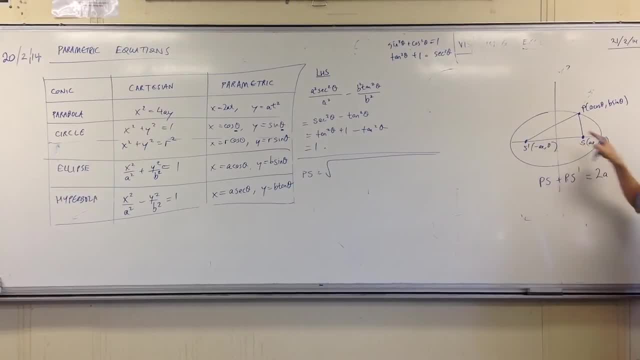 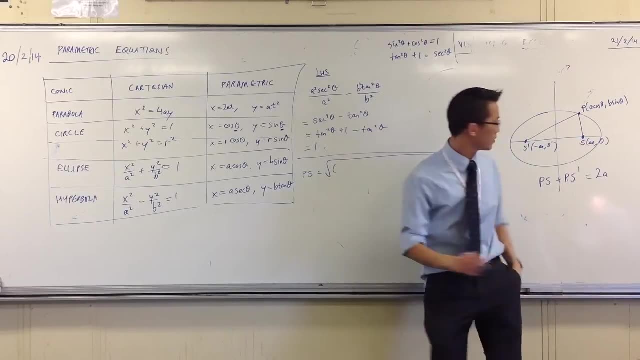 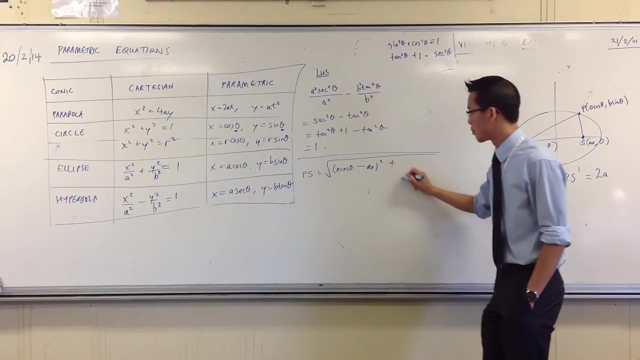 A cos B sin, and I'm going to just do this case, and then the other one follows, very easily. Okay, What's going to go underneath the square root? What have I got? A, I'll do. A cos theta minus. A E squared plus B sine theta minus – because 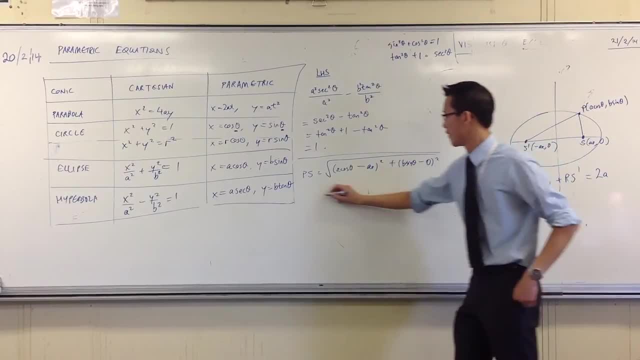 I'm on the axis is just zero, Isn't it Okay? As you look at this, you've got square root of A squared cos. squared equals A square root of A square squared plus B sin theta minus – Б sin theta minus – B sin theta. 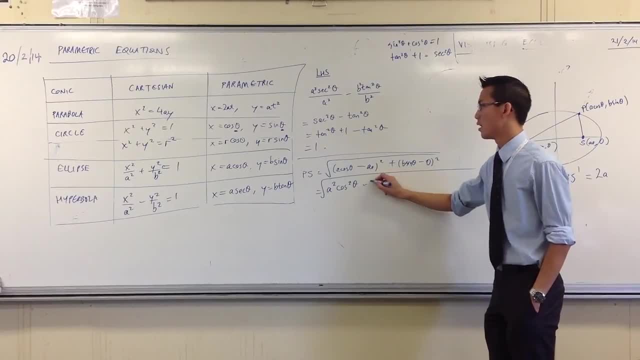 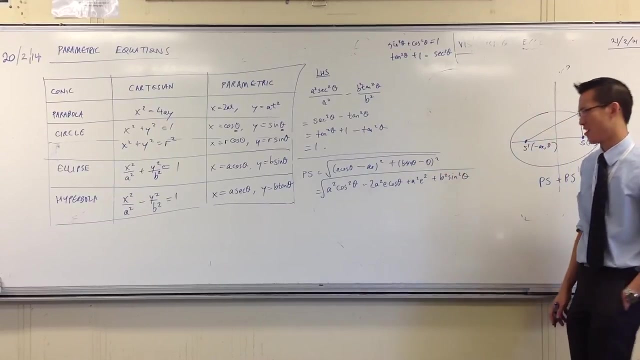 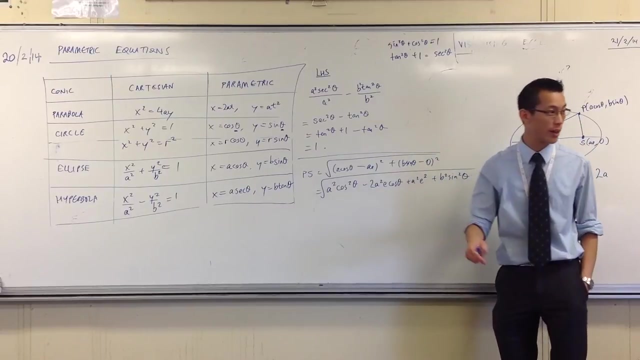 and then their root of square: OK 2, a squared e. cos theta? yes, a squared e squared b squared sine squared. now you're like for real, look at that thing, that's a mess. okay, it's actually not that bad. think about it. you've got so many sine squares and cos squares you're going to. 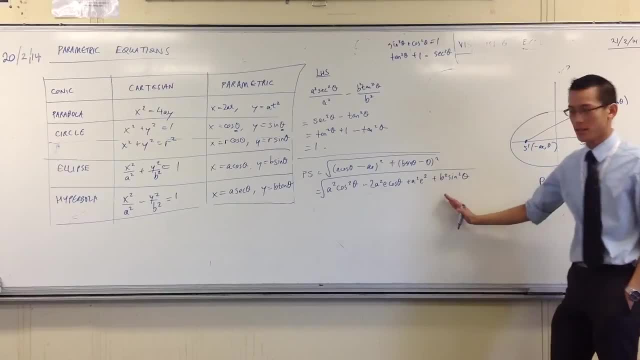 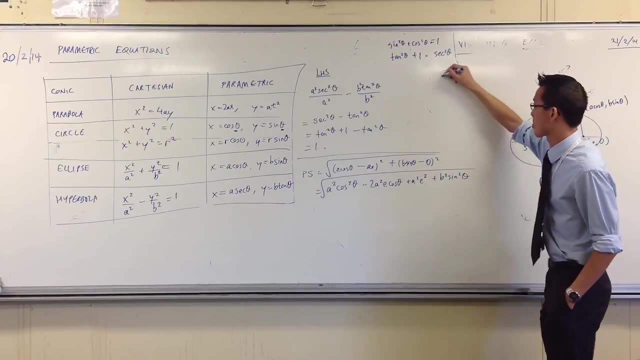 use this guy. okay, you've got A's, E's and B's squared, so you're going to use what's the relationship between a squared and e squared and b squared. remember, come on. we know it by now, don't we? b squared equals a squared for an.